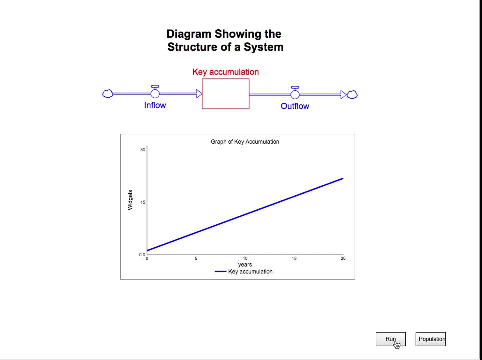 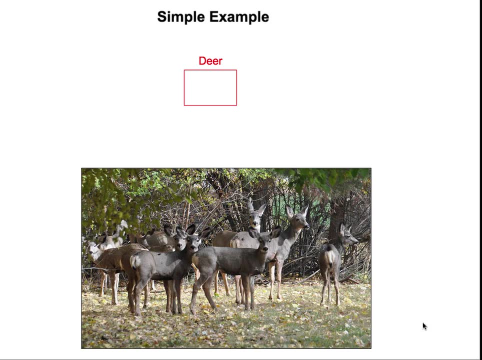 a static picture of a system, but rather it becomes dynamic, like a moving machine or organism. Here's a simple example. Lets say we have a population of deer. The number of deer are represented as the stock. They can be born, adding to the population, and they can die, subtracting from the population. 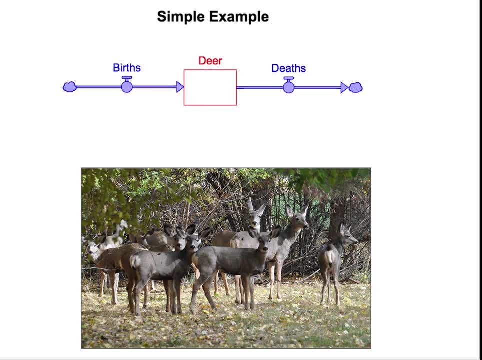 How many are born depends on two factors: how many deer there are and the birth fraction, that is, the percentage of deer that will give birth in any given year. How many die depends on two factors: How many deer there are and the number of young deer that is starting to die, needing birth. 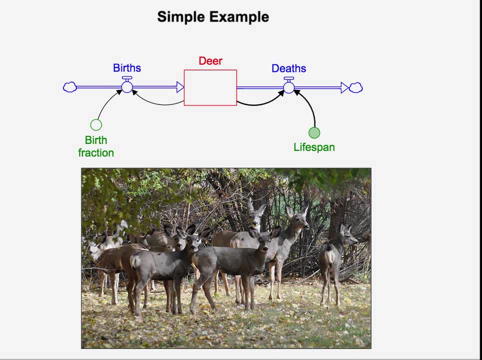 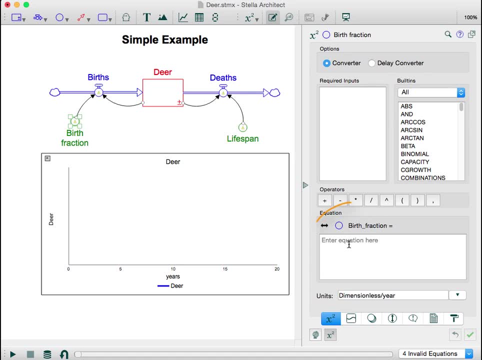 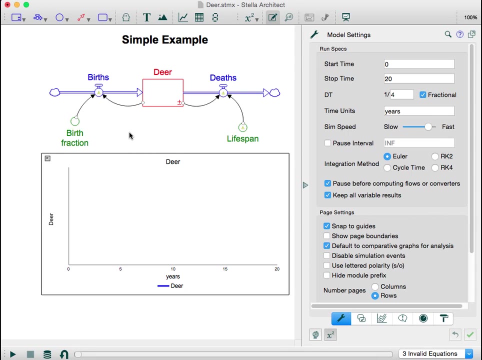 and the average lifespan. To keep it simple, let's say that we'll have 100 deer to start and that the birth fraction will be about 20% of the total deer .2.. That takes into account that about half of the population will be. 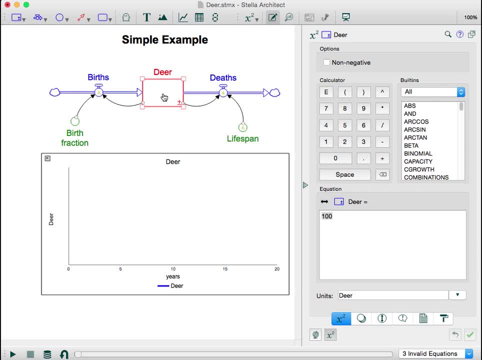 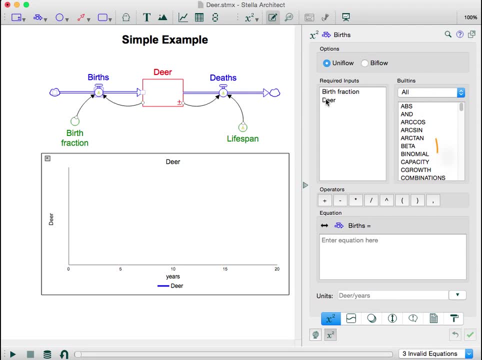 female, and some of those females will be too young or too old to give birth. To figure out the number of births in any given year, we multiply the number of deer by the birth fraction. Again, to keep it simple, let's say the lifespan of a. deer will be about five years. To figure out the number of deaths in any given year, we divide how many deer we have by the lifespan. So on average one-fifth of the deer would die in any given year. Can you guess what we'll have? 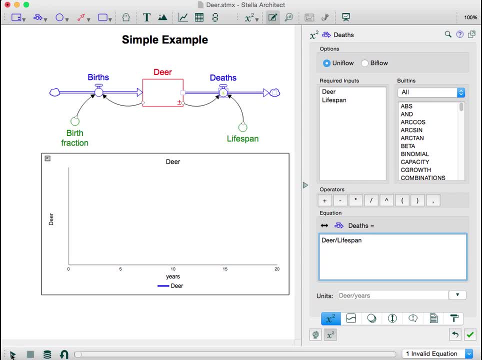 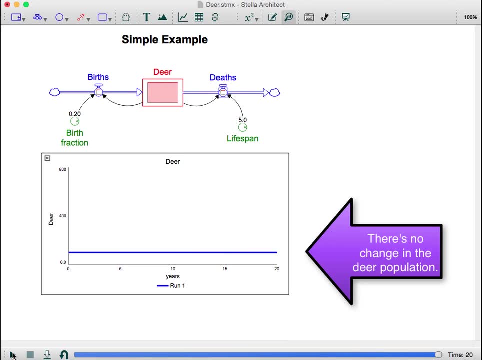 happened to the deer population. given this simple structure and set of rules, Let's find out. Notice that the deer population stays exactly the same for 20 years. Now let's make a simple change. We'll change the lifespan to 10 years. so 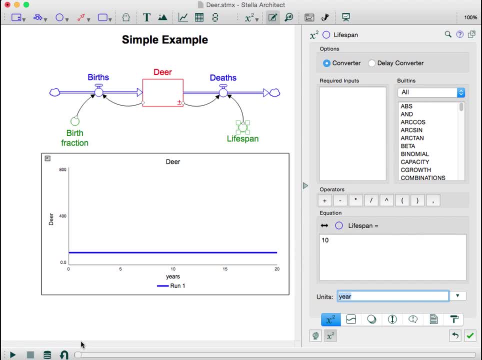 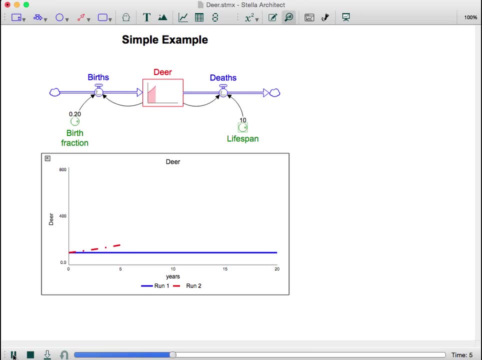 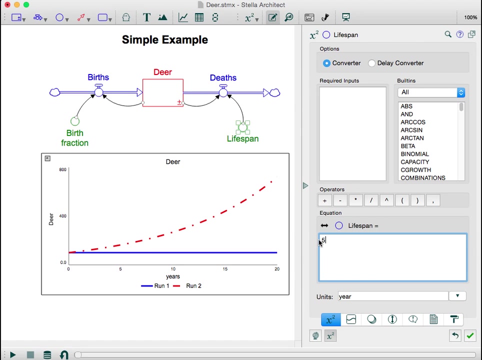 the deer will live twice as long. What do you think will happen to the deer population, Even though the birth fraction is the same? more deer are born because fewer deer die. This allows the population to grow over time. Let's try one more option. We'll reset the lifespan back to five years and then